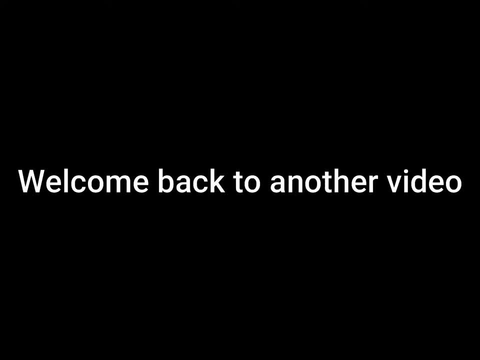 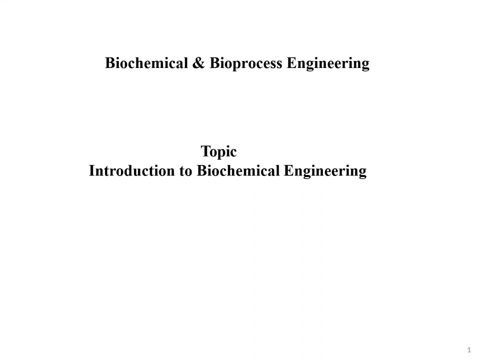 Hey guys, welcome back to a new video. So in this video we'll be discussing about biochemical and bioprocess engineering, which is a new topic for biotechnology. So we'll start off by a little bit of introduction to it and we'll discuss its components step by step. So let's get started. 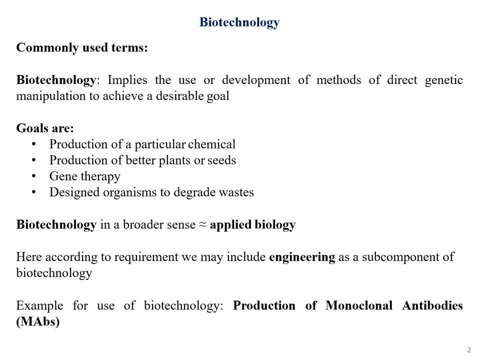 with this. So, talking about this, let's just discuss about biotechnology, first and how, and then how it relates with the subject or the topic. All right, so like the common terminology for biotechnology is, it implies the use or development of methods of direct genetic manipulation to 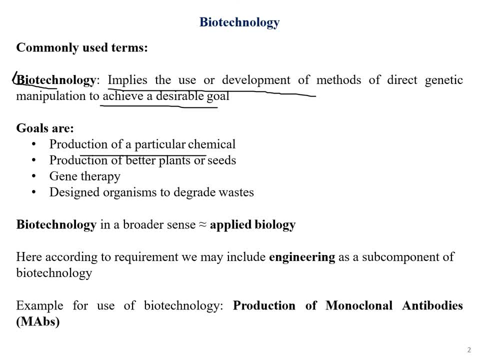 achieve a desirable goal. Also, goals are production of a particular chemical. Goals can be production organisms to repaid waste and biotechnology in a broader sense is, it can be said, as applied biology. Also here, according to requirement, we may include engineering as a component of. 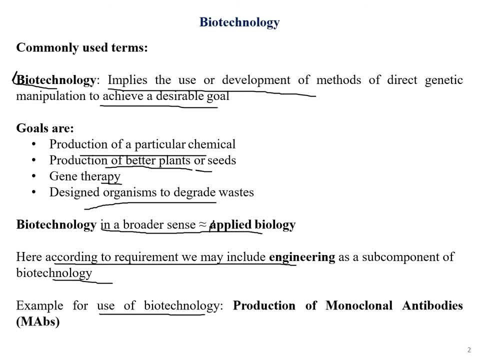 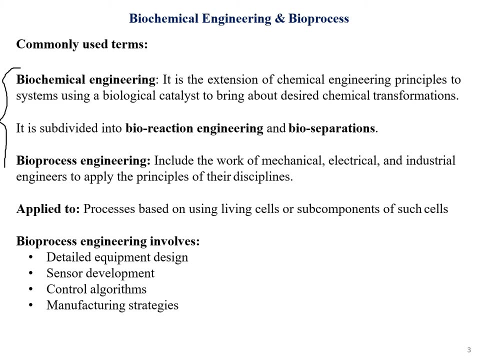 biotechnology. So some of the examples of biotechnology are production of monoclonal antibodies. So I hope you have studied about antibodies or monoclonal antibodies in your junior classes, So we'll talk about each of them. So let's just come to more of the commonly used. 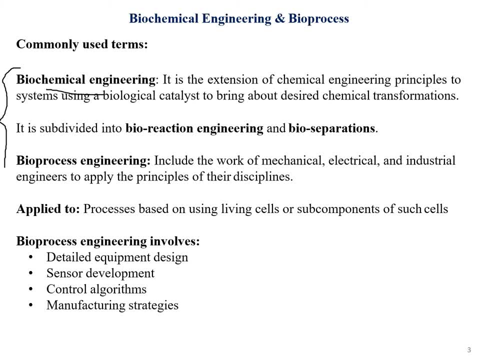 and let's just come to this topic, which is biochemical engineering. So it is the extension of chemical engineering principles to systems using a biological catalyst to bring about desired chemical transformation. So there are reasons why we are using, or focusing on biochemical engineering rather than just simple chemical engineering. All right, so it is. 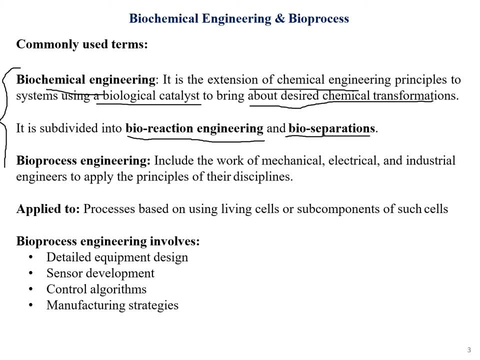 subdivided into bioreaction engineering and bioseparation, Also the bioprocess. the second topic, which is the bioprocess, The bioprocess engineering includes the work of mechanical, electrical and industrial engineers to apply the principles of the disciplines. So basically it's a. 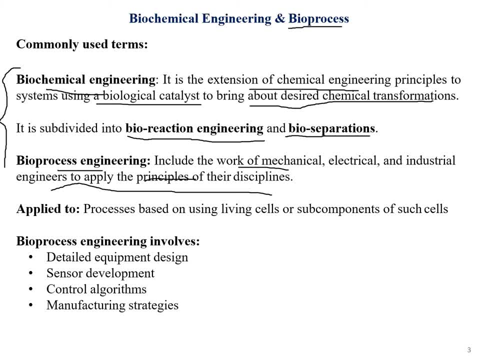 blend of chemical engineering and making of certain things. So we'll just talk about how it. how it has sorts of utility- utilities such as it has detailed equipment design, it has sensor development, it has control algorithm as well as manufacturing designs. Also, it is applied to 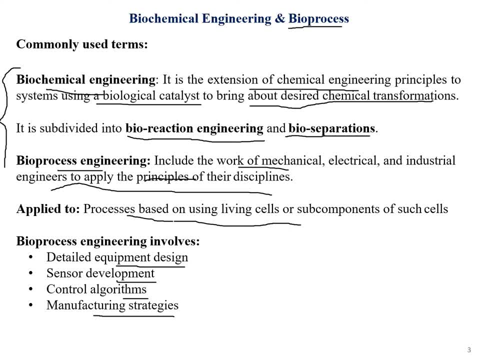 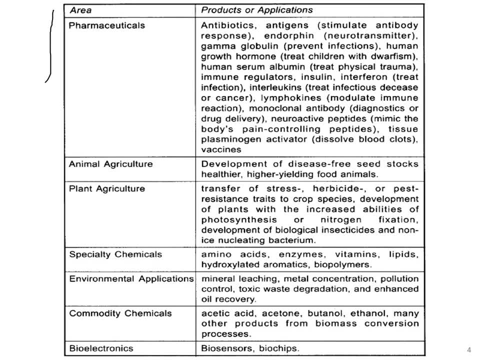 processes based on using living cells or components of such cells. So later in this video you'll understand the usage of the subject and more of its components. So let's. there are lots of areas under which the subjects plays a huge part. So these are areas just pharmaceuticals, and it has. 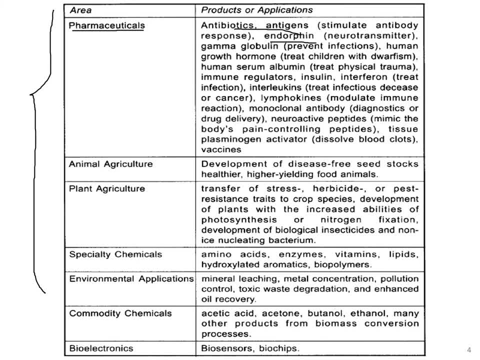 products, applications like antibiotics, antigens, endorphin, gamma globulin, growth hormone, human serum, albumin, immune regulators, insulin, interferon, lymphokines, interleukins. So coming to the second area, which is animal agriculture, which includes development of disease-free seed stocks. Also plant agriculture, which has transfer of 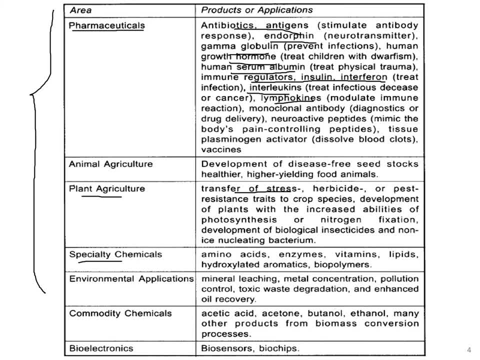 stress, herbicide or pesticides. Coming to the fourth type, which is speciality chemicals, which has amino acids, enzymes and vitamins, and many more. Also coming to environmental applications, it has mineral leaching, metal concentration, pollution control, toxic waste degradation. Coming to commodity chemicals, it has acetic acid, acetone, butanol and bioelectronics as bio. 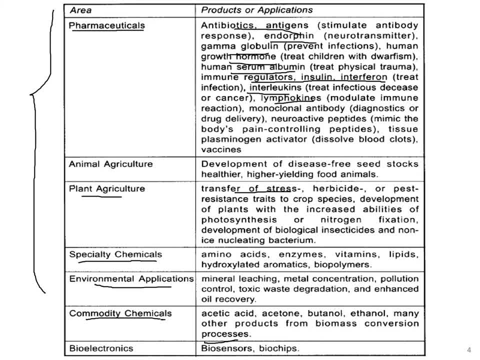 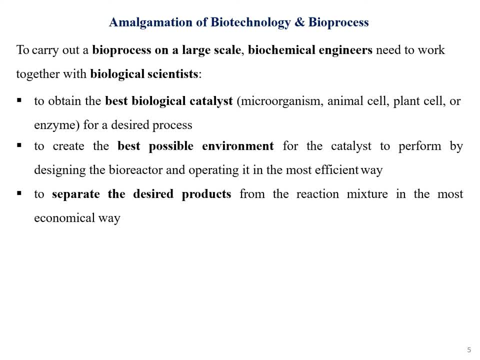 sensors and bio chips. So it has a lot of usages. as you can see With the next part, which is the amalgamation of biotechnology and bioprocess, how it is useful. So to carry out a bioprocess on a large scale, biochemical engineers need to work together with biological scientists, So it is due. 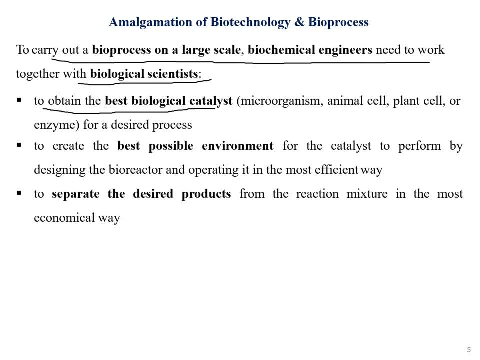 to following reasons, such as to obtain the best biological catalyst, which can be microorganisms, animal cells, plant cells or enzymes for desired process. Also, to create the best possible environment for the catalyst to perform by designing the bioreactor and operating it in the 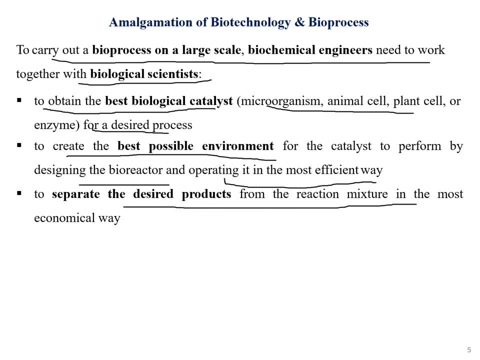 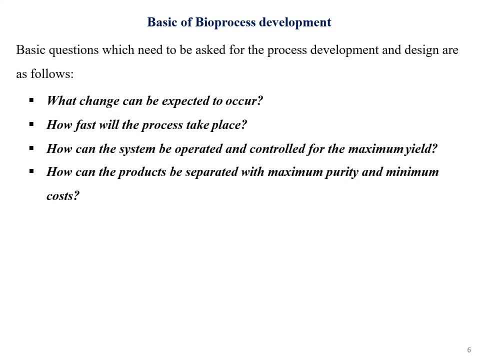 most efficient way. Also, to separate the desired products from the reaction mixture is the most economical way. So it's a blend of two. as you know, it's the bioprocess and the biochemical engineers and bioprocessors. So these are some of the basic questions that might come in your mind. 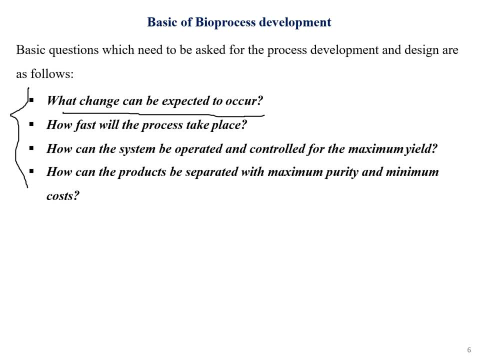 Alright, so these are some of them, such as: what changes can be expected to occur? how fast will the process takes place? how can the system be operated and controlled for the maximum yield? So these are some of the questions that I wrote on this thing, so that might may occur on. 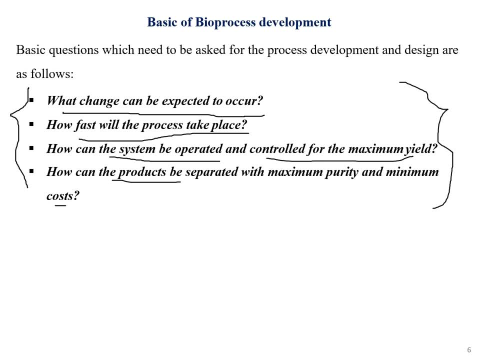 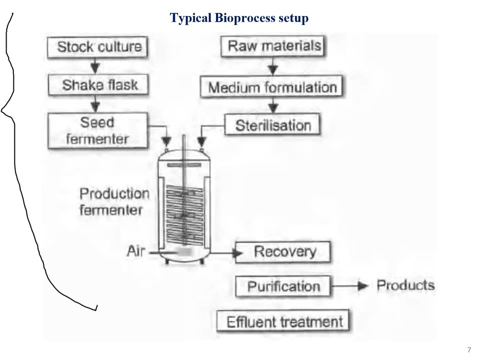 your mind. So I will be discussing about all of these questions and how these questions are. these are the pillars for which we are studying the subject. all right, so moving on. uh, talking about the typical bioprocess setup. so this is a setup. this is the overview of a setup. it has lots. 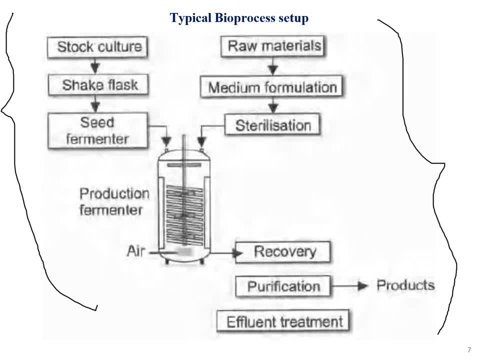 many, a lot of many parts in it when we look interiorly, so on as a looking on as an overview. it has a stock culture, it has a shake flask, it has a seed fermenter and goes into this and it is a main fundamental, it is a production fundamental. this is the air input and this 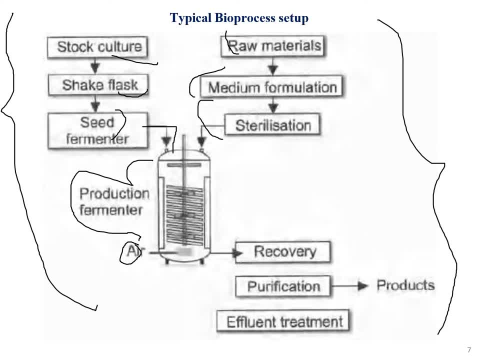 has in the other side. it has raw materials, medium formation, formulation, stylization, and from there we get the recovery product which needs to be purified. so we get the product and the remaining waste is the effluent treatment. this is a basic overview of the bylaw. a bioprocess setup, so moving. 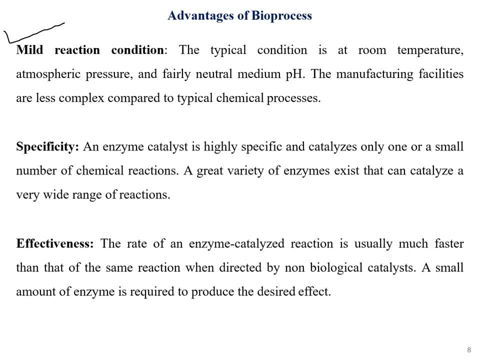 on. so, like coming to the main part, uh, to one of the most important part, which is the advanced of the bioprocess. so how it is advantageous. so it has mild reaction conditions. so the typical condition is at room temperature, atmospheric pressure and fairly neutral ph. the manufacturing. 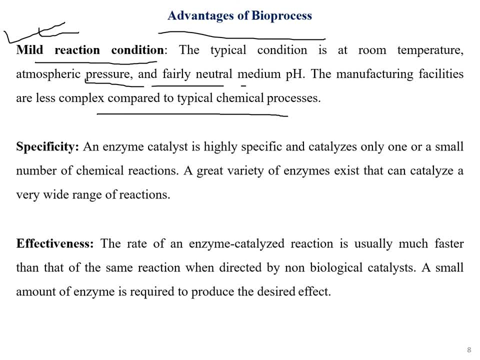 facilities are less complex compared to typical chemical process, so it is. so, basically it happens on a normal scale, so it does not require extremes of temperature or pressures or anything. so it happens on a very gentle, uh, fairly normal, uh, temperature, pressure, neutral, ph scale. so to come into the second advantage is the specificity. so an enzyme. 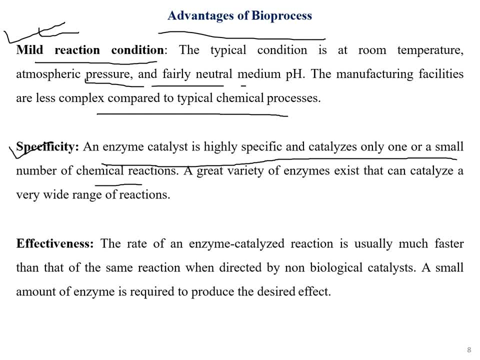 catalyst is highly specific and catalyzes only one or small number of chemical reactions. a great variety of enzymes exist that can catalyze a very wide range of reactions. so here comes the main part of the use of enzymes. so you'll, in this subject, we'll be using a lot. 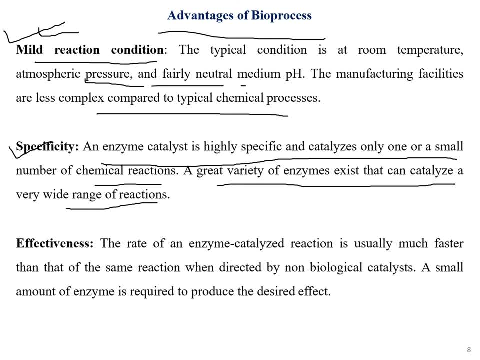 many enzymes and see its activity towards a bioreactor and how it reacts. so there can be many times that exist and can catalyze a lot of a wide variety range of reactions. so here comes the specificity and which helps us to process this reaction better. so, coming to the third part, which 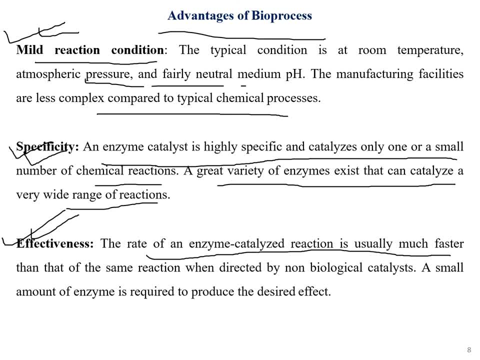 is the effectiveness. so the read of an enzyme catalyzed reaction is usually much faster than that of the same reaction with directed by non biological catalyst. also, a small amount of enzyme is requiring required to produce a desired effect. all right, so this is a pretty much good. 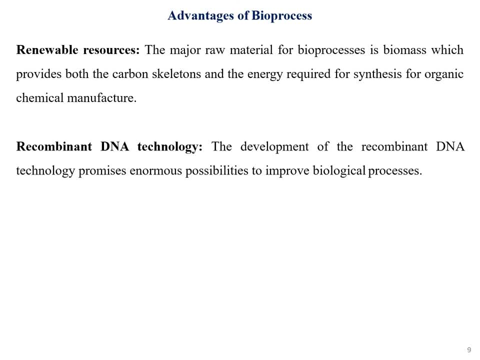 uh good, uh, pretty much efficient, i must say. coming to more of the advantages, such as the renewable resources, so the major raw material for bioprocesses, biomass, which provides both the carbon skeletons and the energy required for synthesis, for organic chemical manufacture. also, usage of recombinant dna. 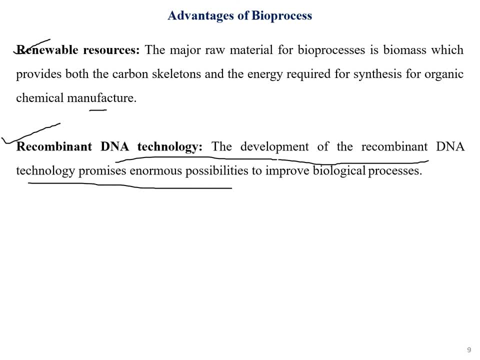 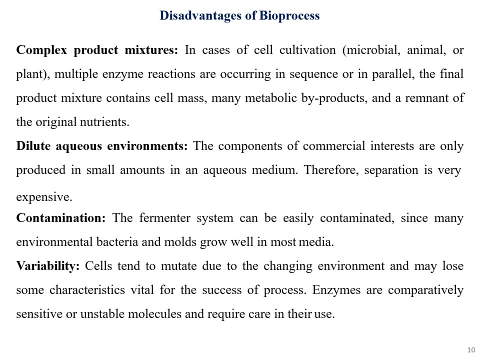 technology. the development of the recommended dna technology promises, uh, enormous possibilities to provide biological processes. so these are some of the advantages as so, as we went through the advantages, there are equal number of just that. we need to go through and understand the entire thing to get the entire context right. so, coming to the first, 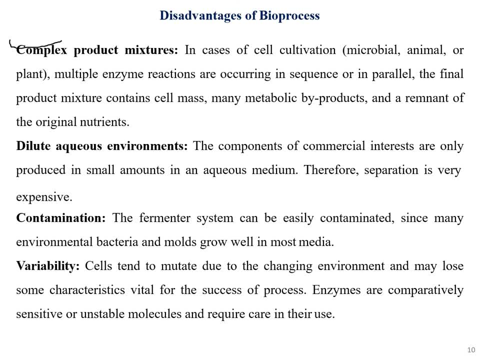 disadvantage of bioprocess, which is the complex product mixtures. so in cases of cell cultivation multiple enzyme reactions are occurring in sequence or in parallel. the final product mixture contains cell mass, many metabolic byproducts and the remnant of original inside nutrients. so it has a complex uh product mixture. it does not have a simple. 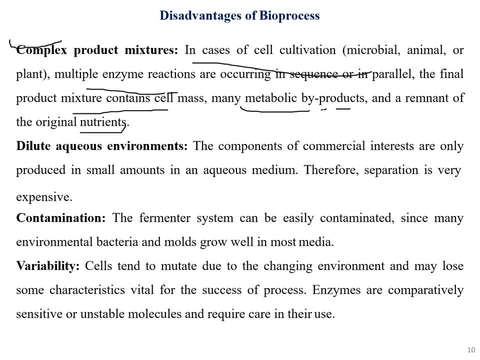 product mixture, so that acts as a disadvantage of this process, sometimes also come to the daily or dilute aqueous environments. so the components of commercial interest are only produced in small amounts and in an aqueous medium. so therefore, separation of separation is very expensive. all right, so coming to the third one, which is contamination, which is the most important. 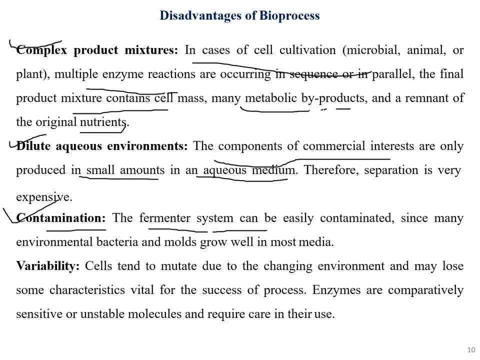 part for any bio processing action. so the thi fermenter system can be easily contaminated, since many environmental bacteria and molds grow well in most media and coming to variability, which is cell tends to mutate due to changing environment and may do some characteristics vital for success or process or enzymes compared. 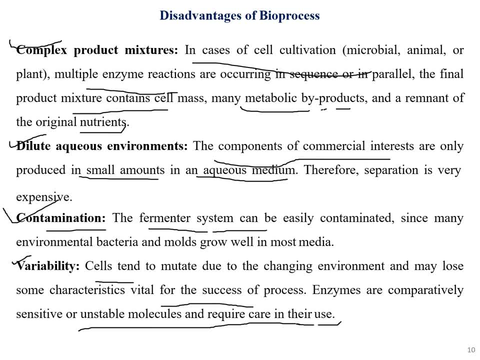 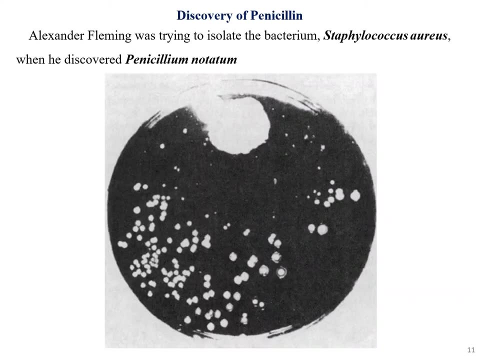 comparatively sensitive or unstable molecules and required care in the use. so variability is another important factor, as cells tend to mutate and now and then, so it's important that we preserve their characteristics. so moving on with. so let's talk about the discovery of pencil and how the process of bioprocess helped in it. so alexander framing was the first person who tried. 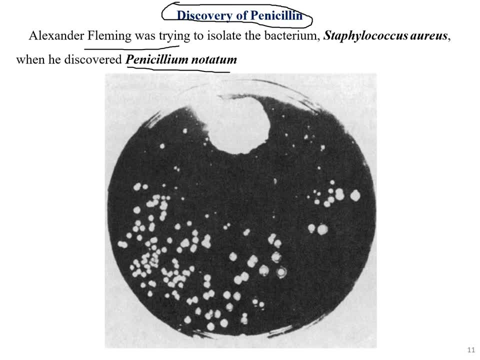 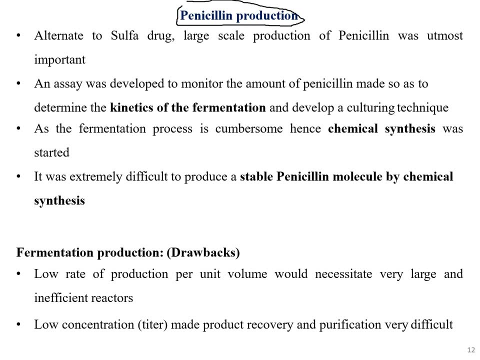 to isolate the bacterium staphylococcus aureus when he discovered penicillin, not atom, both. so the penicillin, uh. so so the traditional or the uh, very old school penicillin production is- was altered to sulphur drugs. sulphur drug is something that is not very mature, uh, in fact it's hazardous for. 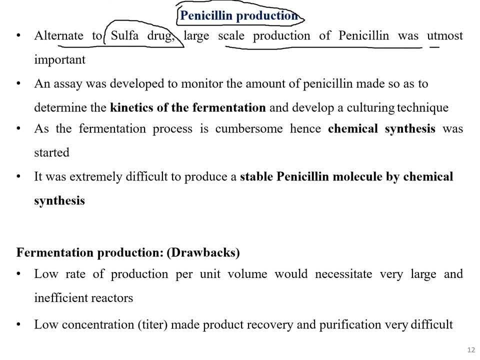 human health. so last large production of penicillin was utmost important. so an essay was developed to monitor the amount of medicine made, so as to determine the kinetics of the fermentation and develop a cultural technique. so as the formation, fermentation process is cubism, hence chemical synthesis was started and it was extremely difficult to produce a stable penicillin. 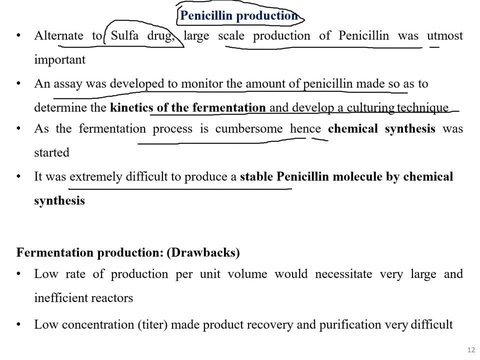 stable penicillin molecule by chemical synthesis. so this was a very much a traditional method for producing penicillin via fermenting things and making up its bigger process. so it has some drawbacks also, as it had a low production rate and it has a low concentration. 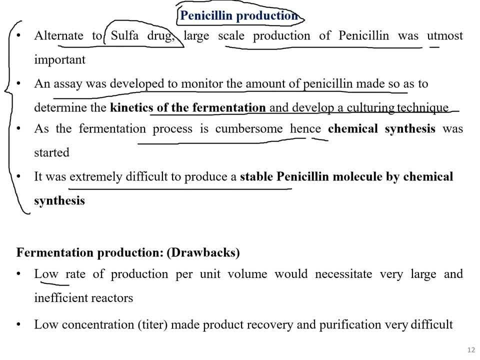 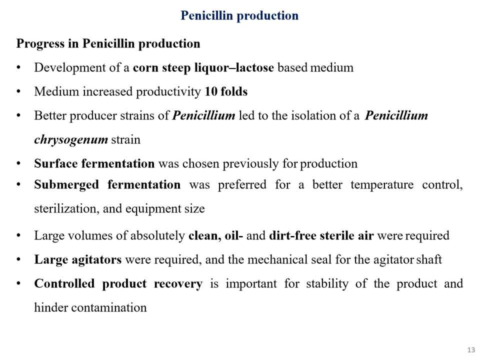 made product recovery and purification very difficult. so, due to low yield, recovery and purification was a major difficulty. coming to the part in which we are, we are interested, so this is the part for bioprocess, so how we plan to develop penicillin and that was a successful 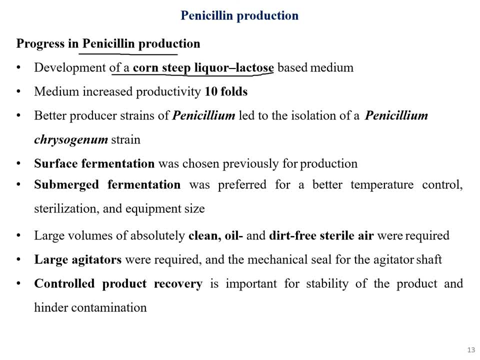 method. so it was the development of a corn steep liquid lactose-based medium and its medium increased productivity 10 folds, so this is a very big plus point. so coming to the next point, which is the eight spread of theingly- all right, are some of the features with penicillin. isolation of penicillin were better producer strains let to the isolation penicillin cryogenomes strain. surface fermentation was chosen previously for production. in this, uh, in this case submerged fermentation was preferred for better temperature control and sterilization. and equipment science and large volumes are absolutely clean, oil and dirt-free, sterile airware required- all right. and large agitators were required and the mechanical sealers seed for the agitator shaft- all right. so these are some of the features for the proprietary phon. 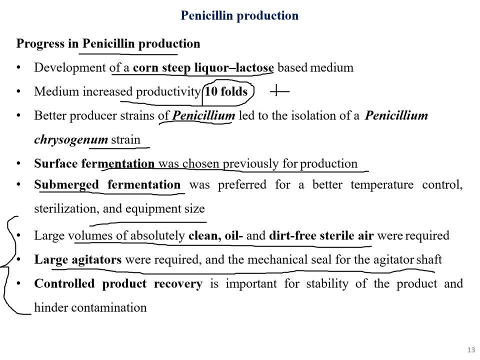 fermenter fermentation, submerged fermentation. It has some of the features involved in it and we'll talk about each of the fermentation in the coming videos. Also, the last point we'd say is that the controlled product recovery is very important for stability of the product and 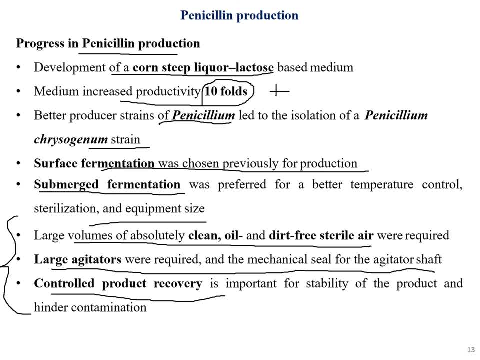 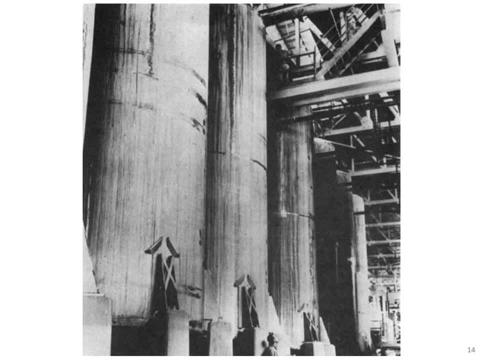 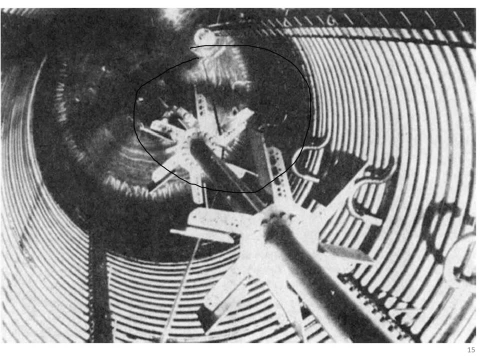 hinder contamination. So this is how, like this is a very general or the advanced technique that comes into play when we apply bioprocess. So this is a picture that I got from Google. This is an outside picture of a fermenter and this is the inward picture of a fermenter. So these are. 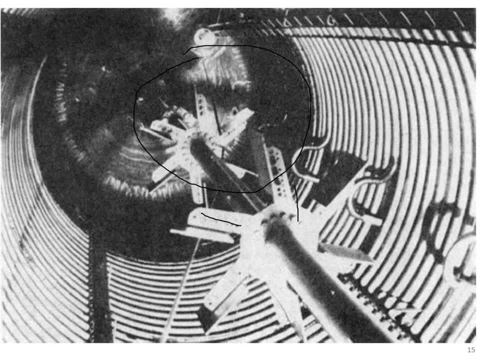 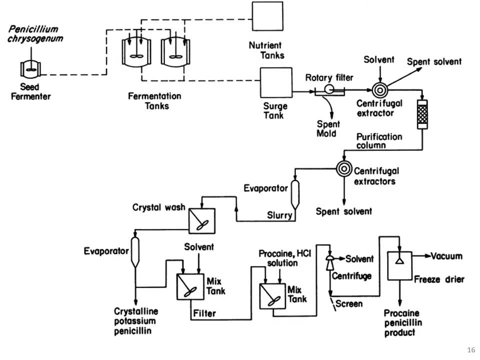 a number of shafts, agitators that help in the formation. So I'll be teaching you about the fermentation deeply So in my coming videos, about what it has and what it doesn't. So this is a basic overview of this thing: how the penicillin is produced in a fermenter. So this is the 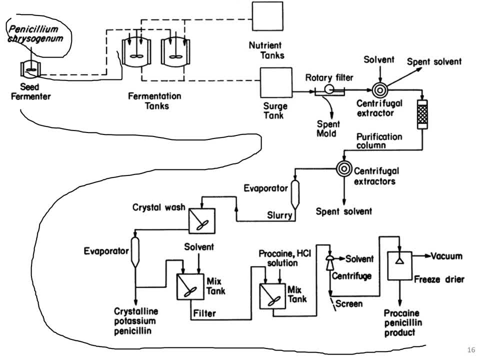 straight penicillin cryogenome and the seed fermenter. So it goes through the fermentation tank. So these are the two tanks and the fermentation tanks are provided with nutrients via nutrient tank. So this is the nutrient tank, which provide nutrient to the both the tanks. 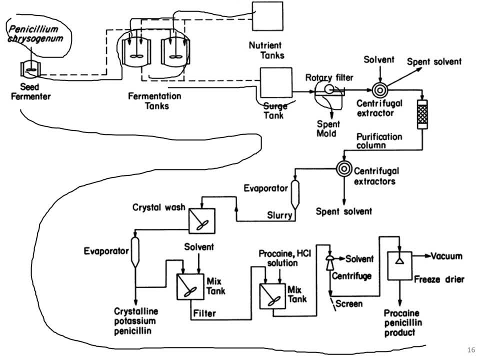 and thus the fermentation tank moves to the surge tank. Here is a rotatory filter and here, through this, it runs the solvent with the help of centrifugal extractor and goes through this and goes through the purification column. Again it runs through a centrifugal extractors.